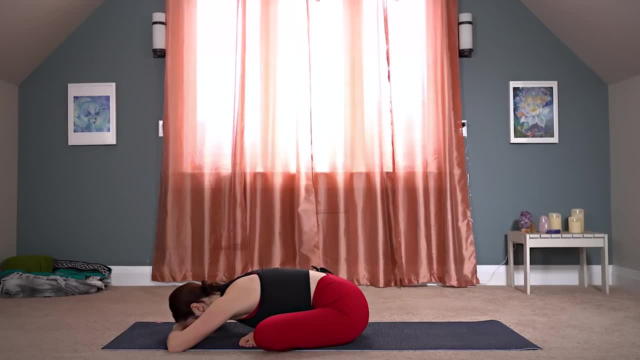 and no matter how far you go into this pose, try to relax your shoulders, relax your chest and imagine you can breathe directly into the spot where you feel this the most. Take one more full, deep belly breath And start to push your hands into the mat, slowly lifting your weight back up to the ground. 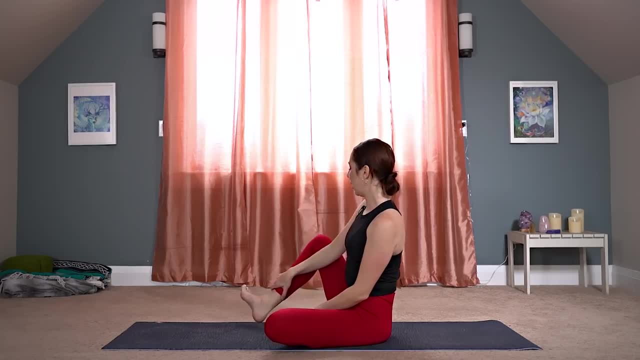 Take one more full, deep belly breath And start to push your hands into the mat, slowly lifting your weight back up to the ground, And from here let's extend our right leg out to the side so you still have your left foot in towards the inner thighs. 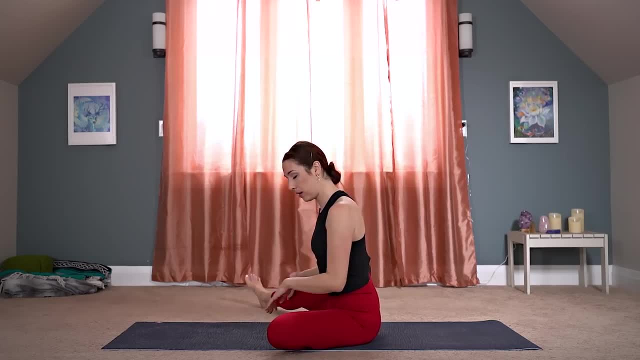 And you can choose where and how much you open both legs away from one another. We're going to start with a side bend. Side bends are so good for our low backs. Reach your left arm up and over, So think of rolling your left shoulder back so you're not. 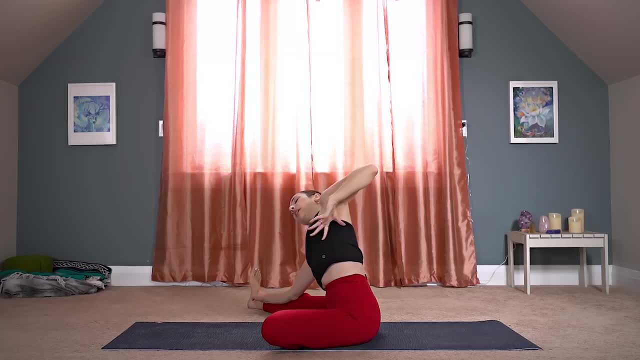 folding towards the floor. This is really more about creating length along the left side of your waist. This is more about creating length along the left side of your waist And see if you can relax your head here. Really stretch out long through your left fingertips. 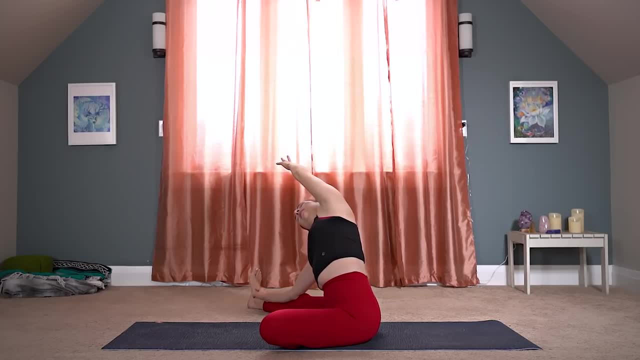 Down that left arm And now looking down towards your right leg. now go ahead and fold on over. So you're folding towards your right leg and your shin. I'm making this a passive fold, meaning I'm letting my spine round, I'm not pushing. 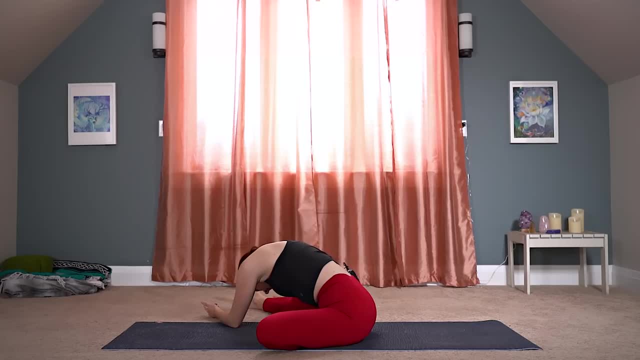 I'm not pulling, just let gravity pull you into it and you should feel a nice stretch along the left side of your lower back. so we are not chasing sensation here. so two more breaths. use arm strength to push into the ground and slowly lift back up. 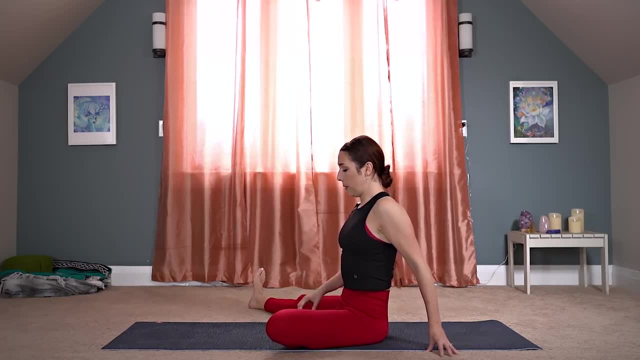 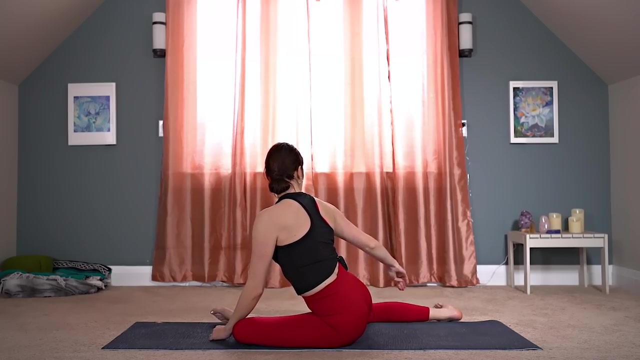 and now from here we're going to find our way into deer pose. so you can just align your left leg. you want your shin parallel to the top of the mat, your left knee in line with your hip and you can send your right leg back. so i have my right knee in line with my right hip and my right shin is in line. 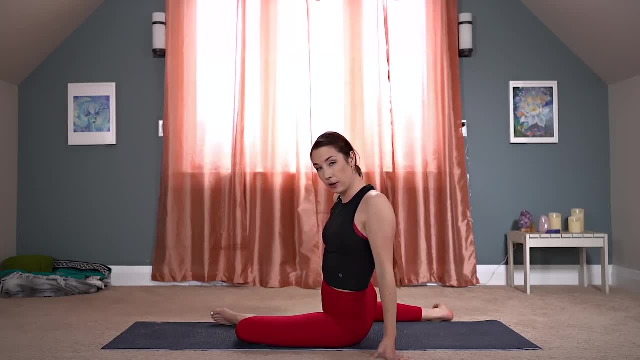 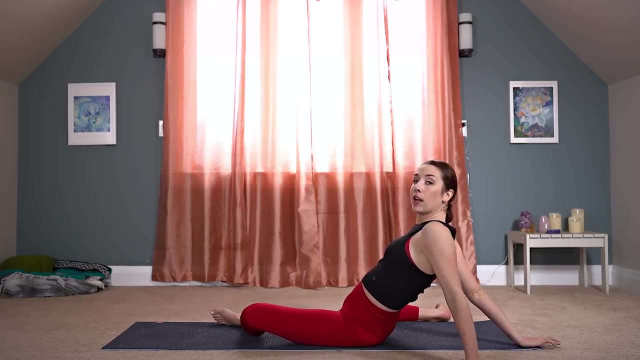 with the long edge of the mat. this is a deep hip stretch for the inner internal rotation. start to walk your hands back as you press that right hip down and you're kind of walking back in a diagonal here. you don't need to go very far in this one. 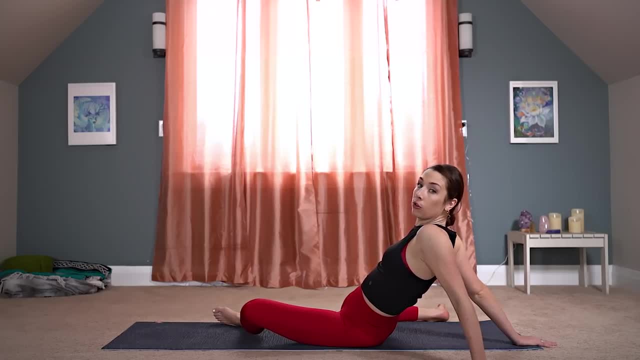 for some people this is very easy and you might be able to lay down directly on your back, but i know for me this is a pretty intense one. we don't do a lot of internal rotation in yoga, so this can get quite tight in a lot of us. 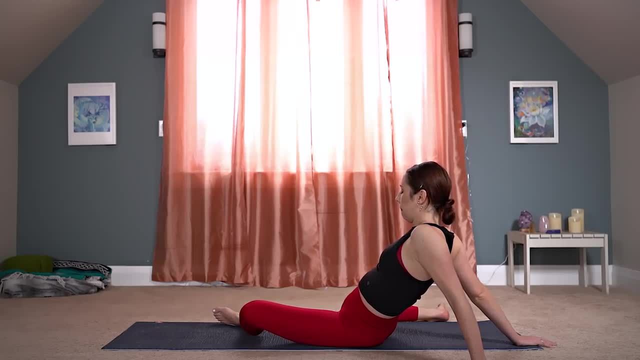 when we work on hip flexibility, we often think about the outer hip, the sides of the hip and into the glutes. but it's really important to think of the hip joint from all angles: inner thigh, front of thigh, outer thigh, the whole thing. and then we're going to use our right hand to push our left foot into the ground. 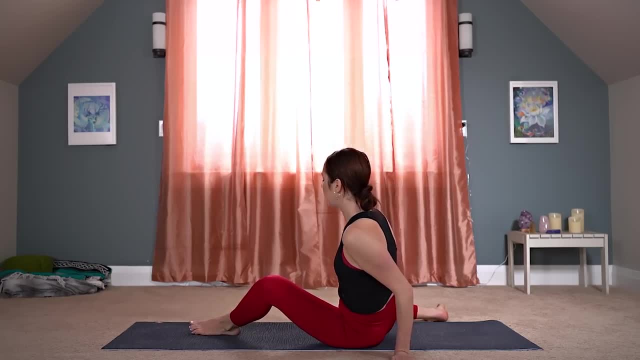 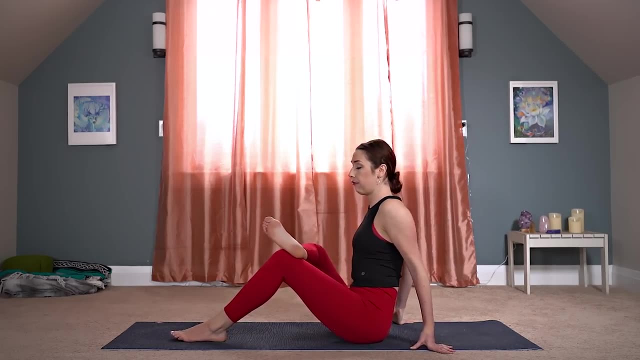 and then we're going to use our right hand to push our left foot up. let's walk our hands back in, lift your chest and one last pose here before we switch sides. you can help that right leg come back, and this time you're going to cross your right ankle. 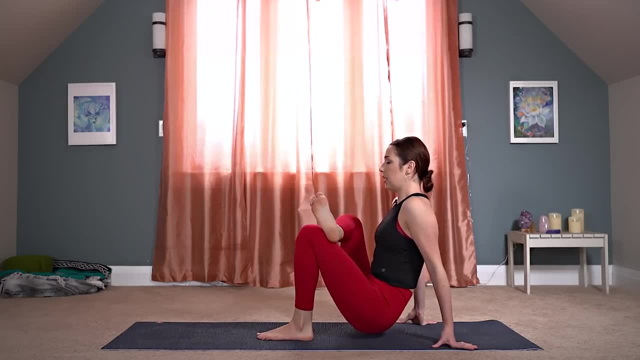 over the top of your left knee for your seated pigeon pose. if the hips are really tight you're going to keep that left leg almost straight. otherwise you can walk that foot in to bring the shin and the foot closer towards you and use your hands to push into the floor to lift your heart up a little bit more. 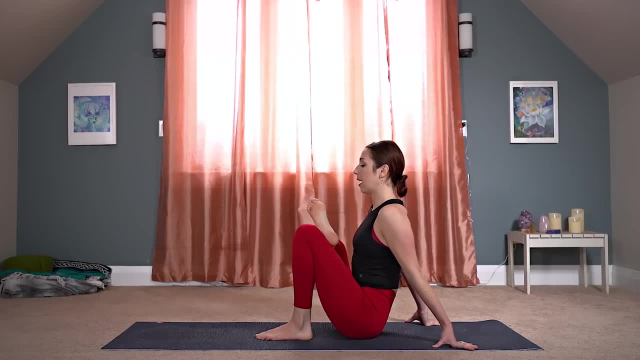 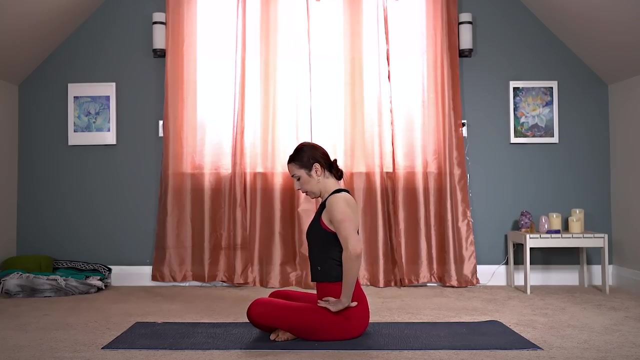 little bit more And I like to just rock a little bit side to side, Press your shoulders down and away from your ears. We'll come into our first pose on the other side. So you want to have your left shin staggered in front of your right one. both sit bones, pressing down, lengthen up through. 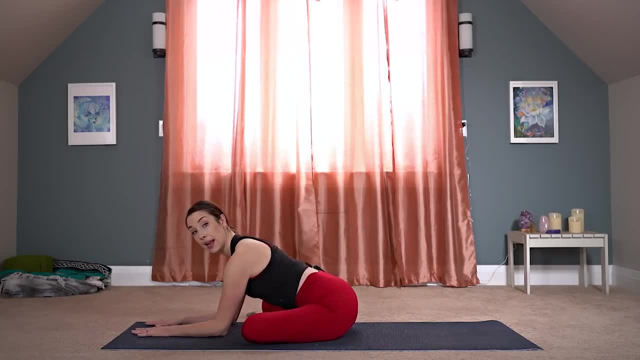 your spine and then start to fold forward, Maybe staying up on your palms, on your forearms, or coming down forehead to the mat or to the back of your hands. Five slow, steady breaths here, Always reminding your upper body to relax. 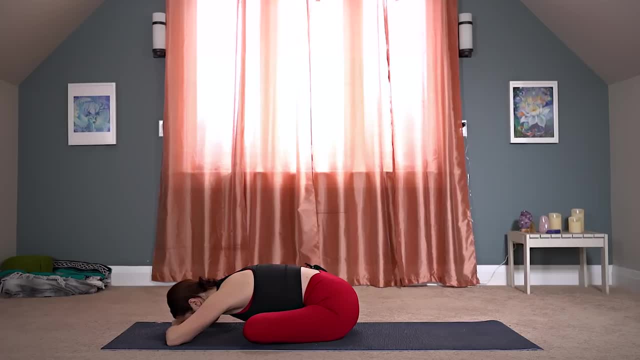 a little more, As if you could breathe directly into your outer left hip. Let's come out of the forward fold, Take your time, Keep your right leg as it is and extend your left leg out to the side. Open up your left leg. 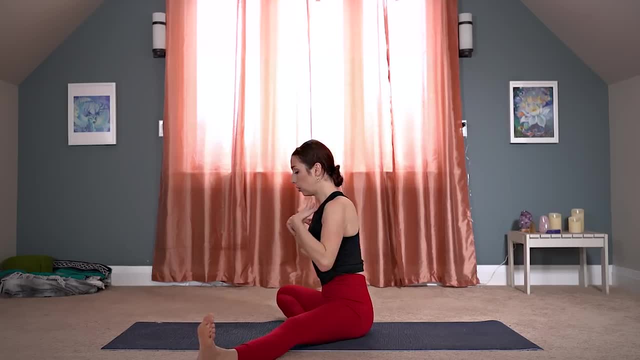 We're going to do the same thing for the other side. So keep your spine lifted, reach your right arm up and over, Roll your right shoulder back As if someone was pulling on your right hand, get a little bit more length and lift through the right side of your waist. 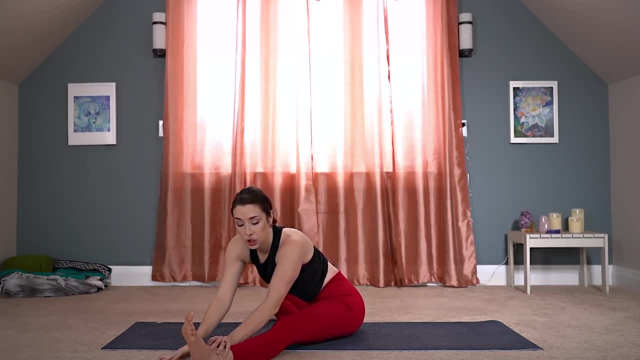 Then you can turn to face towards the floor, towards your left chin, and then fold on down, And I'm turning my palms to face up towards the floor and then fold on down and I'm turning my palms to face up towards the floor. 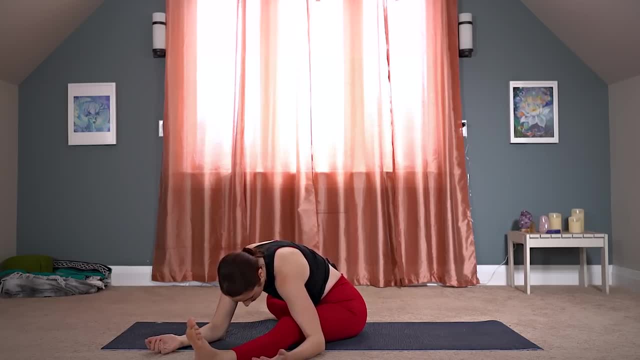 I'm. I'm going to make sure that your arms are still out, So your right hand is still up, and I'm going to pull your hands in to your hips and your hands are still up up towards the sky. I'm not pushing, not grabbing, not forcing my way deep into a 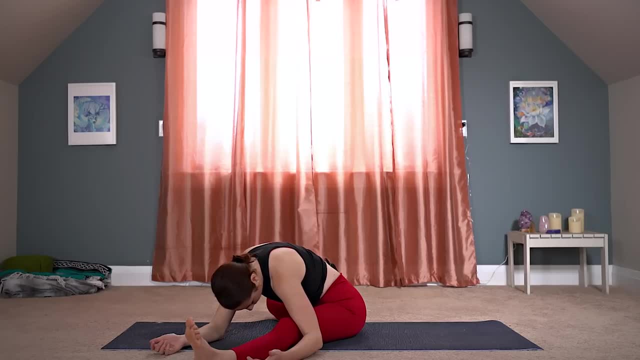 pose, especially when we're working with lower back. less really is more. try not to hold your breath. let's walk our hands in lifting up into our deer. pose on the other side, so you want your right shin aligned with your left hip and then you're going to lift your right leg up. 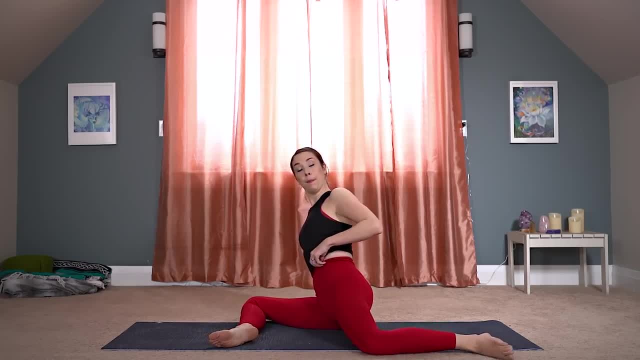 aligned to the top of the mat. your right knee is aligned to your right hip and then you're bringing your left knee in line with your left hip shin to the long edge of your mat, start to press and roll that left hip down as you walk your hands back, kind of in a diagonal. 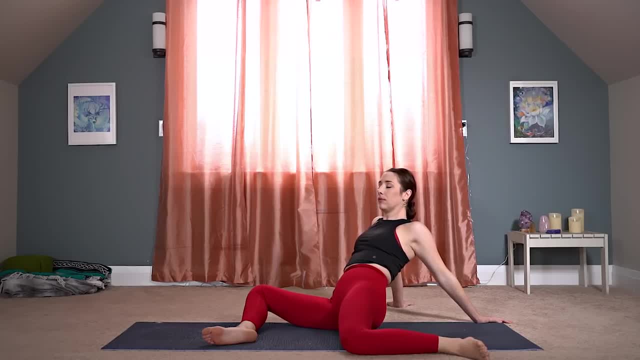 and you might notice that one side feels very different from the other. we're not trying to replicate the exact same experience. it's very, very normal to have asymmetry in your body and go ahead and walk back up our last seated pose into our reclined pigeon so you can bring. 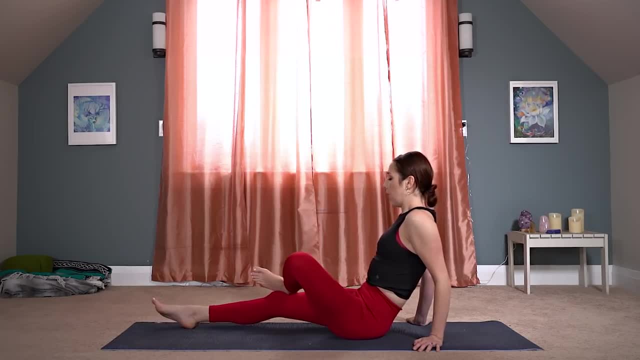 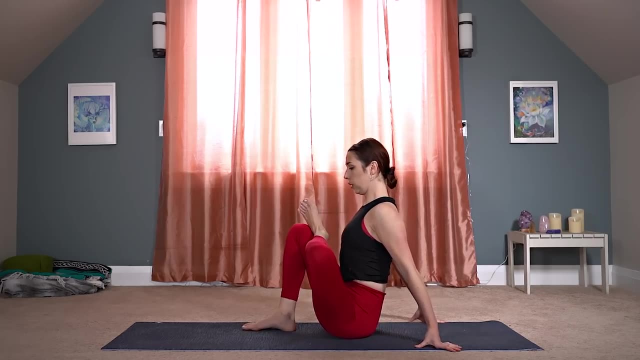 that left leg out in front of you. you're crossing your left ankle over the top of your right knee and bring that right foot in any amount. remember to roll your shoulders down and away from your ears. think of lifting your heart up and maybe rock a little side to side. 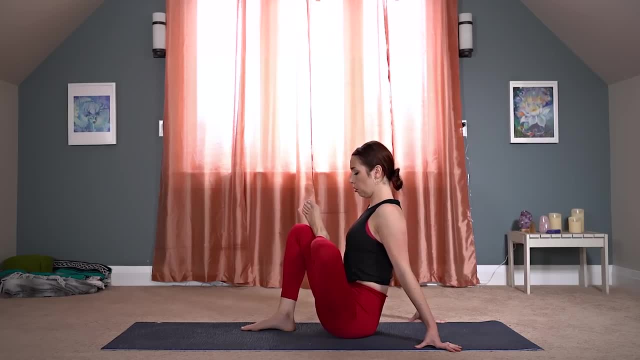 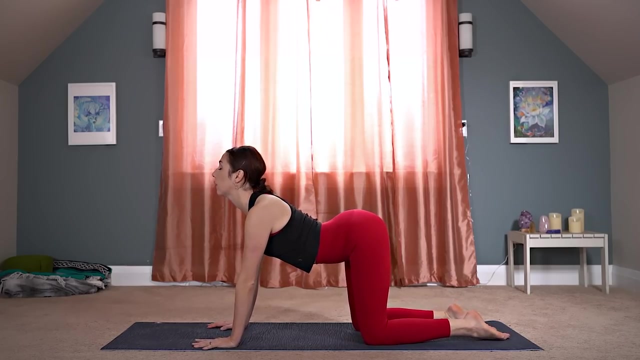 drawing your lower belly in a little and let's release tabletop pose for cat and cow. bring your hands under your shoulders, knees underneath your hips as you inhale, drop your belly, lift your gaze, curl tailbone up, exhale round and contract chin to chest. take a few more here, same thing, going with your breath. 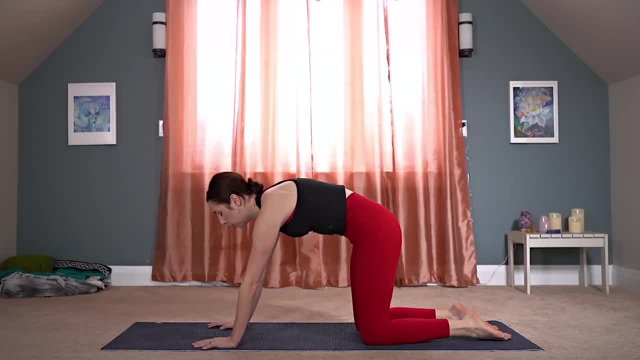 and try to get this motion to flow evenly in your lower back, your mid back and your upper back. you've been stretching a little through your shoulders. take your last one here: inhale, drop the belly, lift the gaze, tailbone up, exhale, push the floor away from you as you round coming. 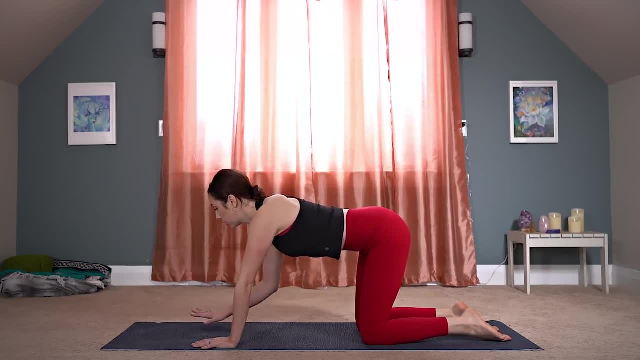 back to neutral. we'll find down dog, but we're gonna do a wider version. so walk your hands out and we're gonna go down dog and we're gonna go down dog and we're gonna go down dog and we're gonna walk your hands out and we're gonna do a wider version. so walk your hands out and then we're. 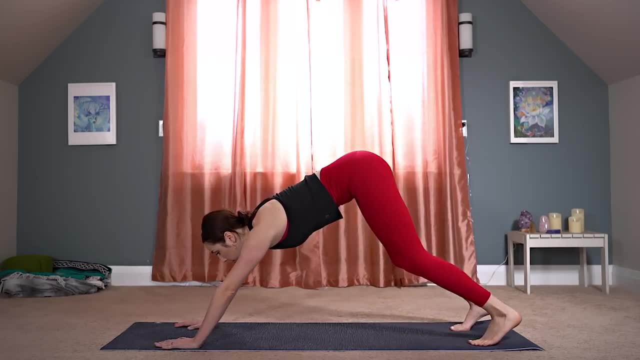 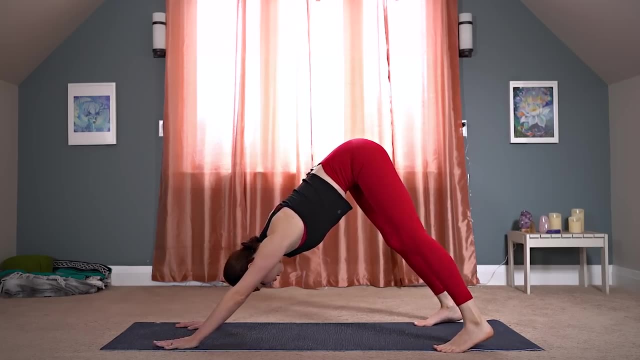 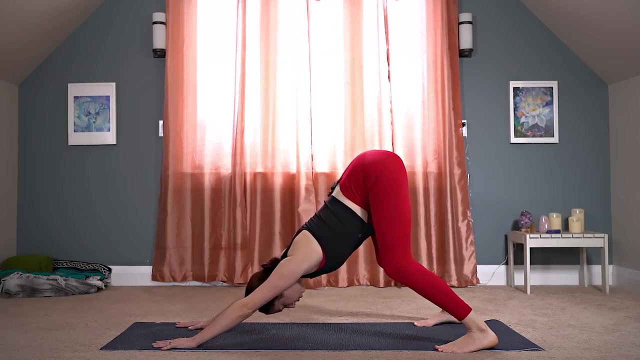 you're going to tuck your toes under to lift your tailbone and your hips up and walk your feet out towards the edges of your mat. so a much wider stance than what we would normally do in our down dog, and you might want to bend your knees generously as you push into your arms and push. 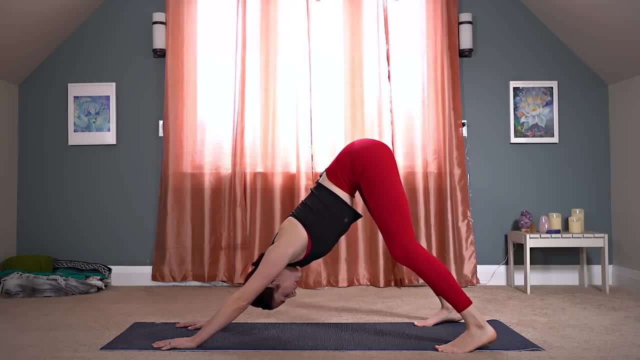 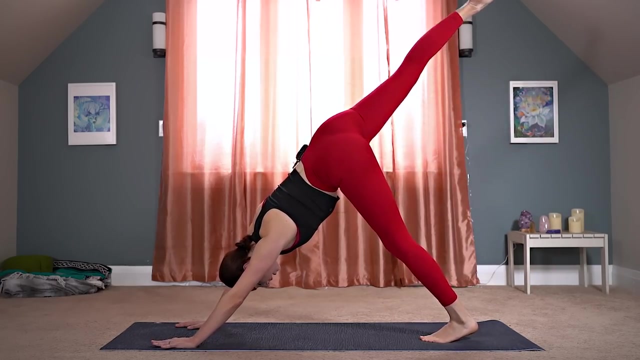 your chest towards your thighs. relax your head, relax your neck, really draw your lower belly in here and now. bend your knees even more, just so you can bring your feet together a little more. so hip with distance apart. let's reach our right leg up towards the sky. bend your right knee open. 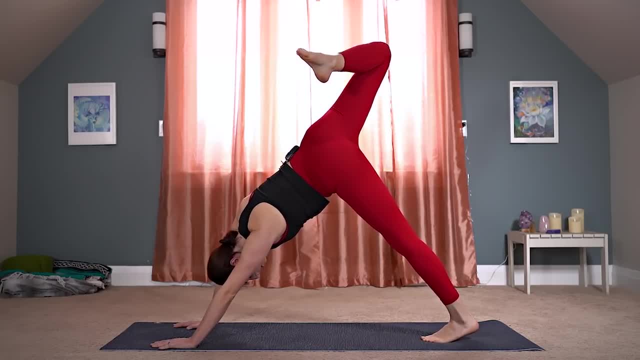 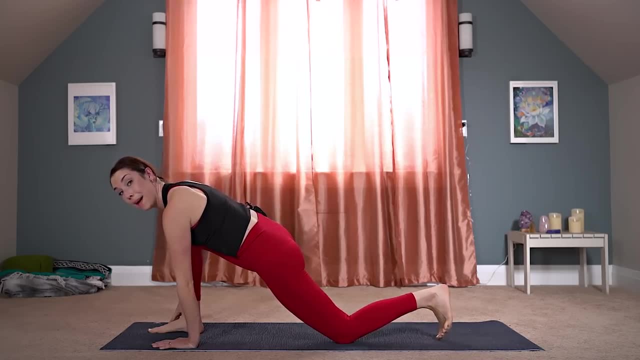 up your hip. big stretch here and we'll step our right foot in between our hands to the top. of the right knee is on top of your ankle. back knee comes down to the floor, adding a twist here. so we're stretching into our hips and then for our low back we're twisting right hand. 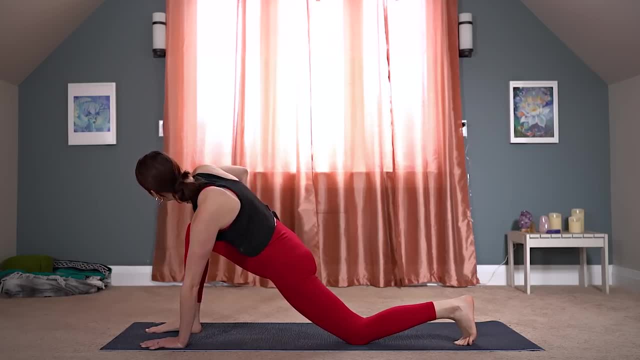 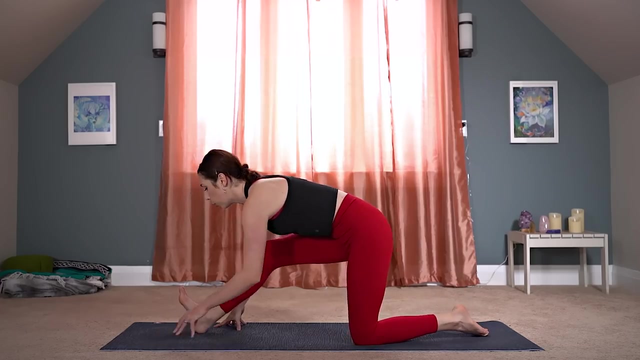 onto your thigh, push your hand into your leg as you roll your right shoulder back and open up through your chest. try to melt your hips forward and down towards the floor, getting deep into the psoas, deep into the hip flexors, looking down to the mat again. start to straighten your right leg and you're welcome to just stay up. 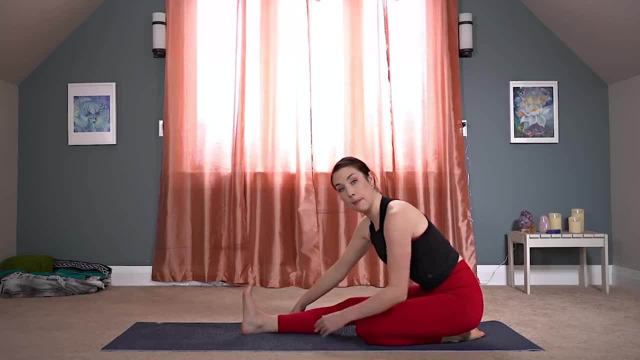 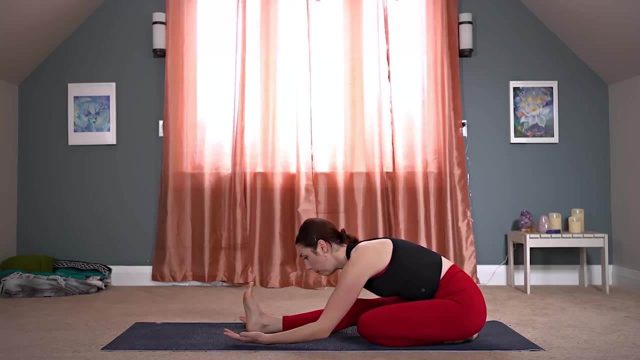 here, or i find it easier to just let my hips come back to sit on my left heel, and then we're going to fold down again. i'm letting myself round here. i'm not pushing, i'm not pulling, and then i'm going to fold down, and then i'm going to fold down again. i'm letting myself round here. i'm not pushing, i'm not pulling. 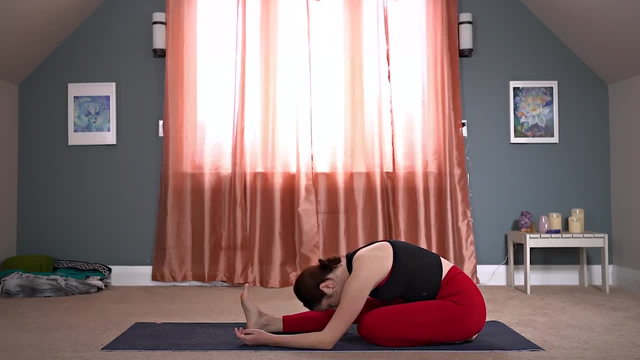 I'm just letting my body come into the version of the forward fold and the depth of the forward fold that is most appropriate, so targeting the back of our hip at the insertion point of the hamstring and stretching along our low back. drop your head and if you had folded down like what I'm doing here, you need to lift your chest. 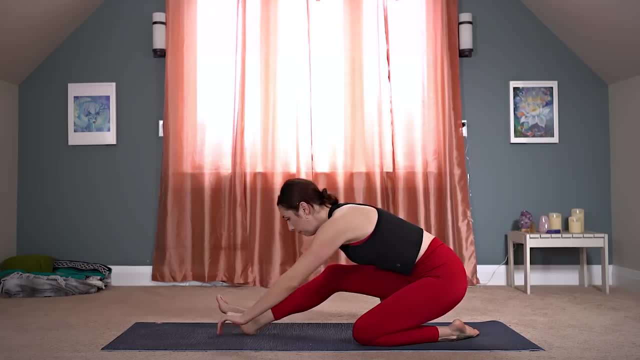 up a little bit. we're gonna bend into that front knee again, coming into a tabletop pose. so we're gonna bend into that front knee again, coming into a tabletop pose. so we're gonna bend into that front knee again, coming into a tabletop pose. so just bring your right knee next to. 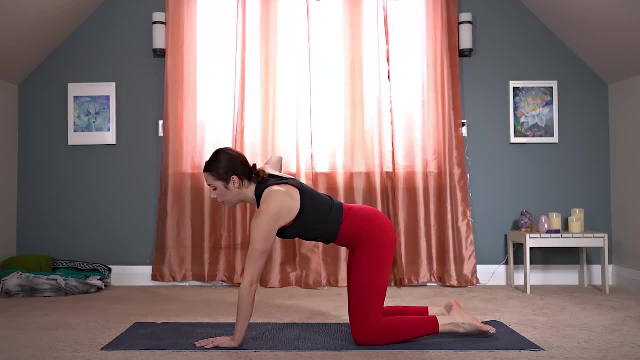 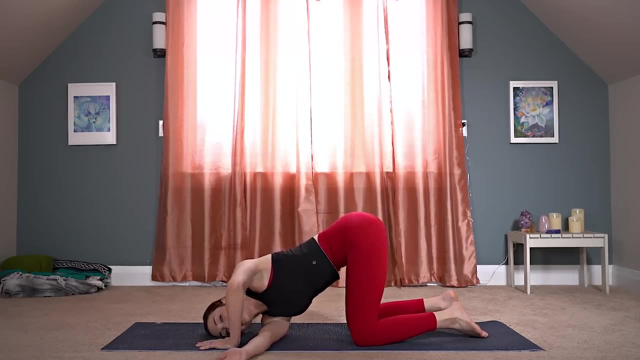 just bring your right knee next to your left, we'll find. thread the needle parashva balasana. thread your right arm underneath you, dropping shoulder and ear to the floor. once you're there, lean a little bit, push into your right hip and you can just push into your left hand. you can also straighten your left. 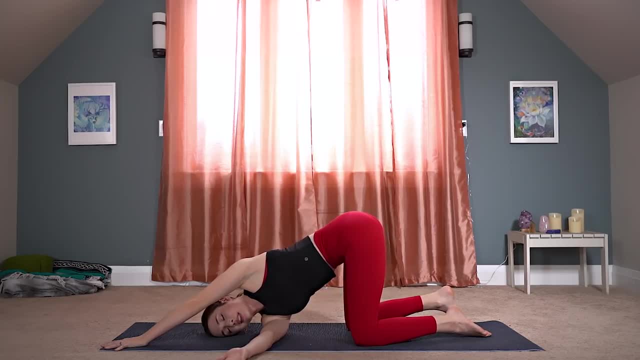 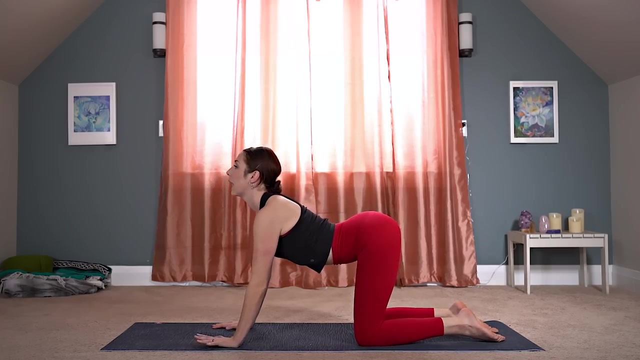 arm up overhead. so just another twist: if you had your left arm straight, slide it back, push into your left palm, come up tabletop pose. it might feel good to take one round of cat-and-cow inhale. drop the belly, exhale round and contract. come back to neutral and we'll find our downward facing dog tucked your toes. 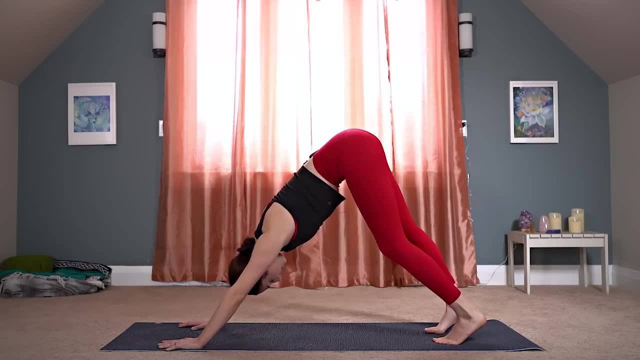 under. lift your hips up and back. you can bend your knees here. second side: let's reach our left leg up to the sky. bend your left knee, open up your hip, really squeeze into your glutes on Janey asana low lunge. step your left foot in between. 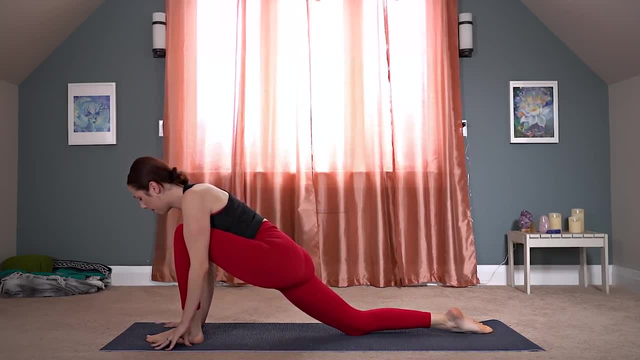 your palms to the top of the mat. back knee comes down to the floor. keep your right hand anchored for support. melt your hips down, bring your left hand to your thigh and really pull your right knee up to the floor. keep your right hand anchored for support, melt your hips down, bring your left hand to your thigh and really. 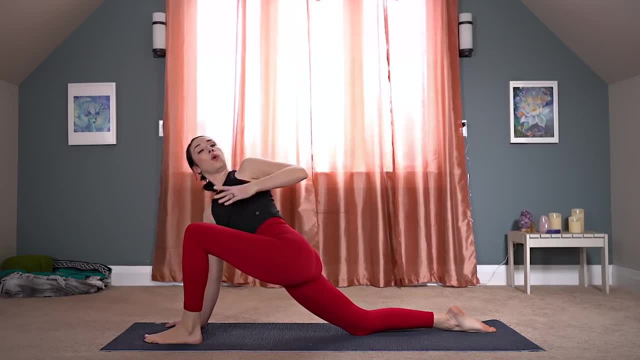 push your hand into your thigh in order to lift and rotate that left shoulder back. let gravity pull your hips down lower towards the floor and, facing down to the mat, we'll find our half splits again. ardha hanumanasana, either staying up nice and high. 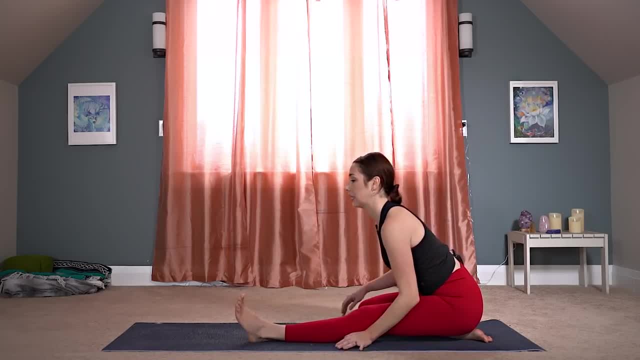 or just letting go, letting your hips rest on your right heel, this time folding forward five breaths in the pose. you can absolutely keep a bit of a bend in that left leg. it does not need to be perfectly straight. you do not need to force your way into any kind of pose. 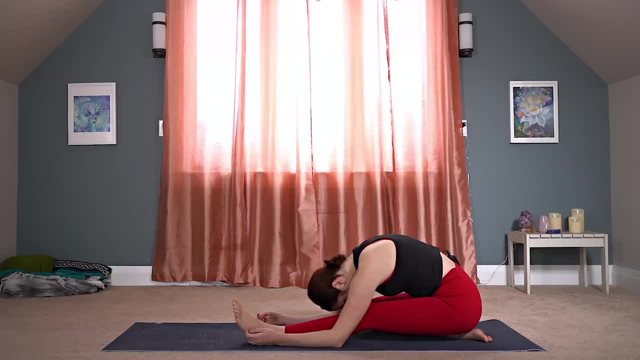 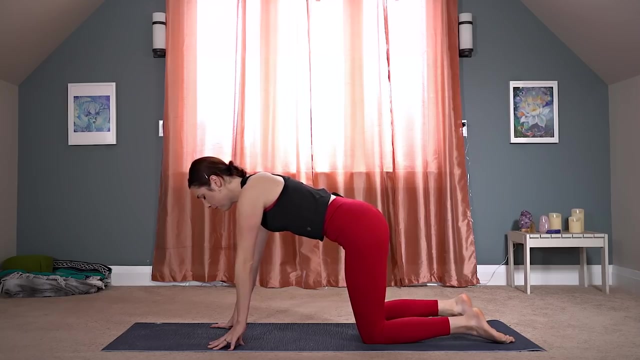 if you had folded all the way down, just lift your head and chest up. we're meeting in tabletop pose for parjva balasana. thread the needle with your knees under your hips. you're going to thread your left arm underneath you shoulder and ear to the mat. 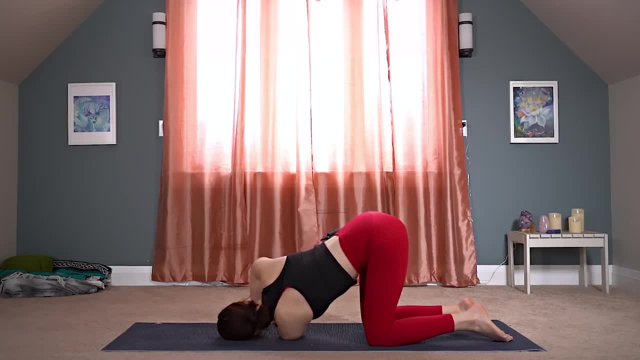 and then you're going to fold your head down to the mat, push into your left hip and maybe keep your right hand pressing into the floor. you can also straighten your arm up overhead, so slide your right hand back down, push into the palm, re-extend up, cat and cow, inhale, belly down, lift your gaze. 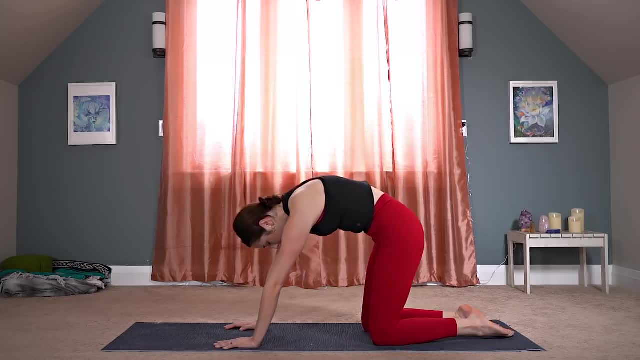 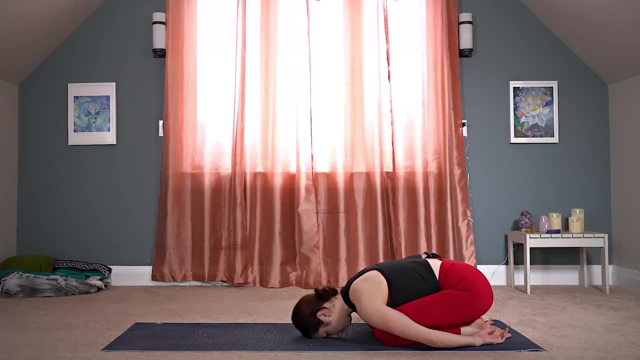 exhale round and contract and just push back into a child's pose. balasana, your arms can either be out in front of you or you can bring your arms back behind you, palms facing up. take a few breaths here. take a few breaths here. 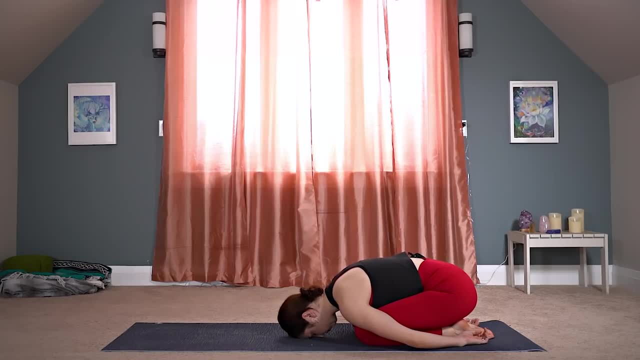 don't make it too deep. hold, continue and then once again breathe, inhale. you can rise up. we're just gonna lay down on our backs, so bring your legs out in front of you, get ready, you can come on down. ananda balasana or happy baby pose. 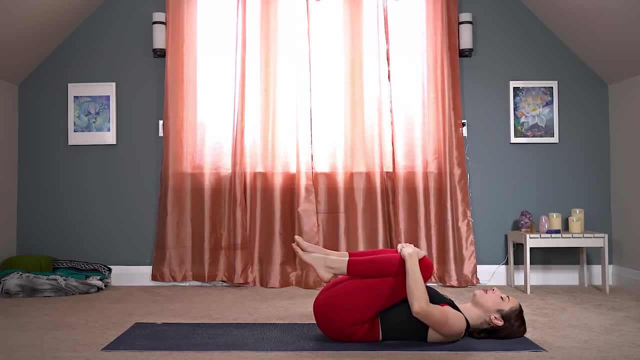 start by bringing your knees in towards your chest, and then you can widen them towards shoulders and armpits, armpits pulling down onto your thighs. This might be enough for your hips and for your low back, but if you'd like to go further, you can grab a hold of your feet or your toes and stack your. 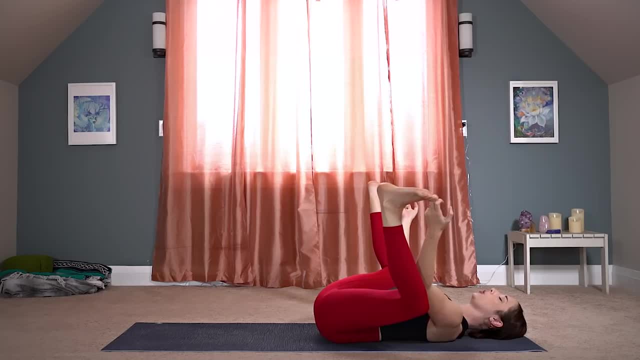 ankles over your knees. Elbows can push open into your thighs a little bit, maybe swaying a little side to side. Remember, if it's too much, just keep your knees bent. Don't worry about holding onto your feet. This is meant to be a therapeutic practice for hips and low back. 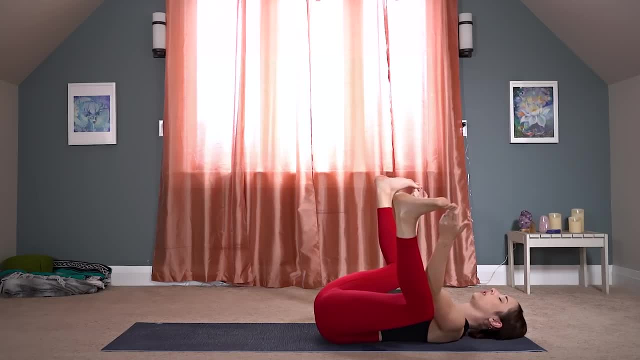 so there's nothing to prove. We're not trying to make things super intense. So Release from this pose Setu Bandha Sarvangasana, which is just a bridge pose. Feet come flat to the floor with your knees bent. Really, shrug your shoulders down and away from your ears. palms face up towards the sky. 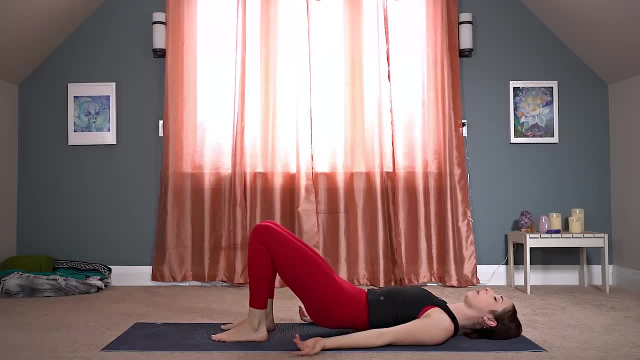 You want to feel your feet push into the floor. curl your tailbone up and start to lift your hips low back and mid-back off the floor. Hug through your inner thighs a little bit, so you're actively pushing into your big toes. 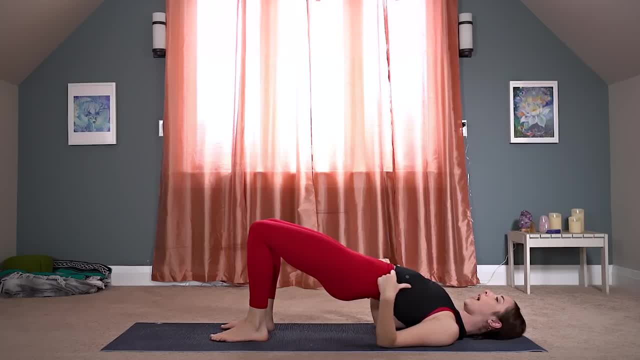 Think of digging down into your heels and dragging them back towards your shoulders. You're going to feel your hamstrings, your glutes and your low back engage, which is exactly what we want. Press your pelvis up a little bit higher. 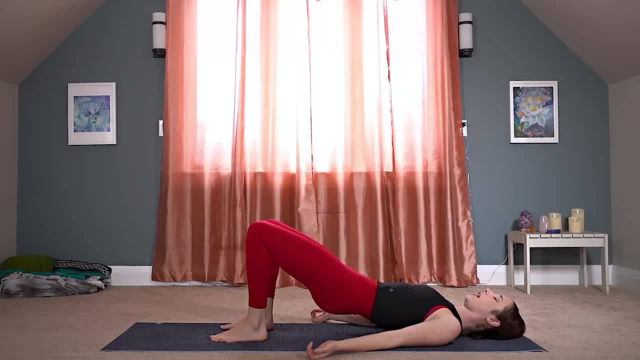 One more big breath And exhale release inch by inch. Let's cross our right ankle over the top of the left knee: Reclined Pigeon Pose- very similar to what we did at the beginning of class. But we're going to do it again. 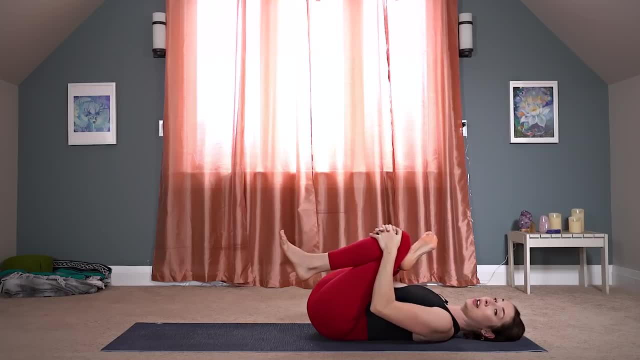 You can go ahead and reach back as you pull that left knee in. This is your first option. if you'd like to also add a hamstring stretch, You're going to straighten your left leg and pull from here. Give it one more big breath here in the stretch. 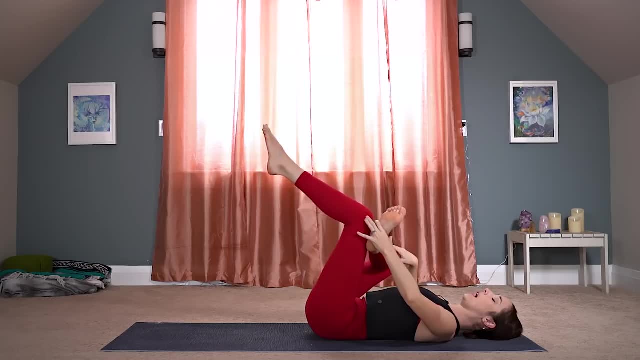 And if your left leg was straight, bend into your knee And you're now going to over-cross. So really wrap your right thigh over your left one, trying to stack your right knee on top of the left. Just a moment here in Shoelace Pose. 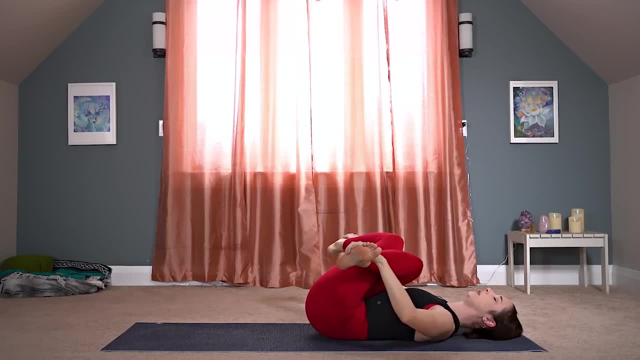 See if you can hold on to your feet as you pull them down, Getting deep into the outer hips, And we'll find a Lange Spinal Twist. So keep your legs as they are. Let your left foot come flat to the floor. Open your arms out into a little cactus shape. 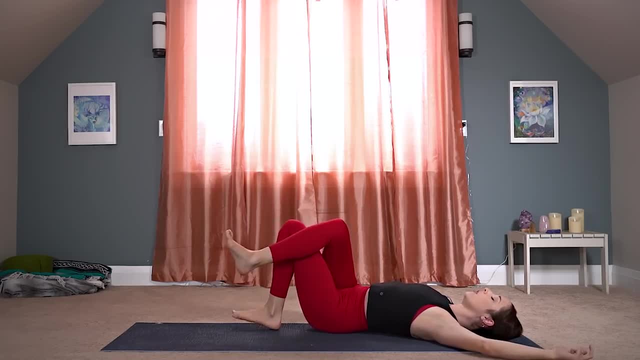 And you might want to lift your hips and move them to the right so that both knees and thighs can drop down to the left. Try to keep your right shoulder pressing on the floor And, if it feels like too much, to have your right thigh crossed like this, 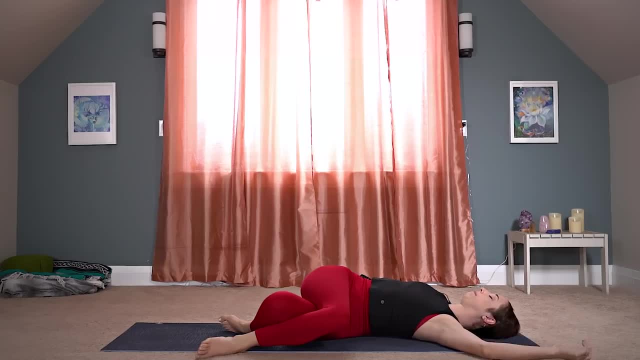 you can uncross them and just have one leg over the other And rise on up with your knees. Uncross the legs. Bring your feet flat to the floor, knees bent. Relax your arms down, Bridge Pose again. Push into your feet. 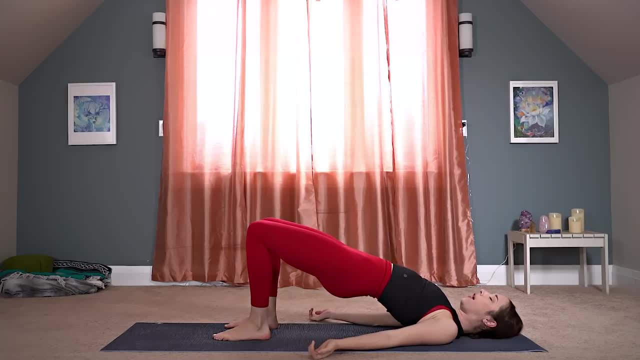 Squeeze your glutes and lift up. Hug through your inner thighs. Push down into your heels and drag them back towards your shoulders. Lengthen your tailbone away from your lower back, as if you're trying to flatten out. Relax your lower back. 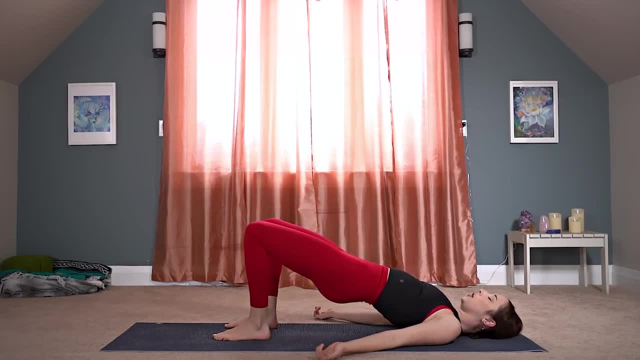 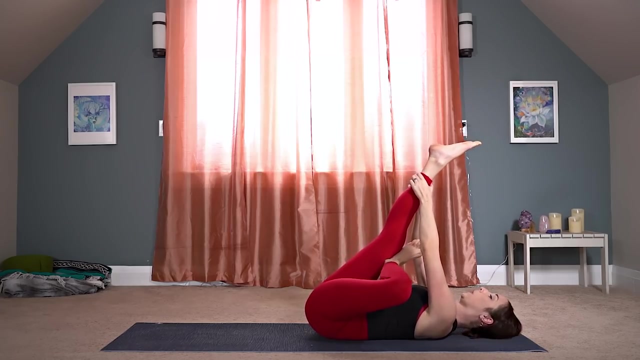 One more breath here And we curl down inch by inch, Reclined Pigeon, Cross your left ankle over the top of your right knee And reach through with your arms, either holding here or straightening your right leg And reaching up a little bit higher towards your ankle. 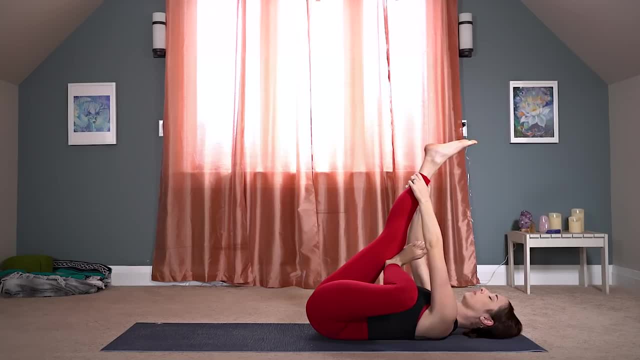 Escaping Pigeon. One more Squeeze: Bend your right leg, Shoelace Pose, so wrap your left thigh over your right. one, reach for your feet or whatever you can grab a hold on. we're not here for very long, you're just pulling down and 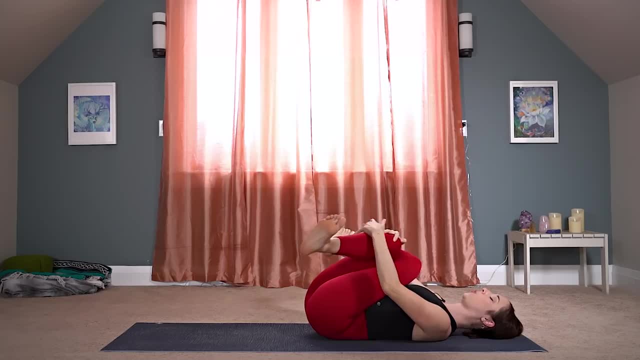 moving your feet away from one another. you can also just hold on to your knees and pull them in this way and let's release into our laying spinal twist, open up your arms. you can move your hips over to the left. both knees and thighs drop down to the right. push down into your left shoulder. 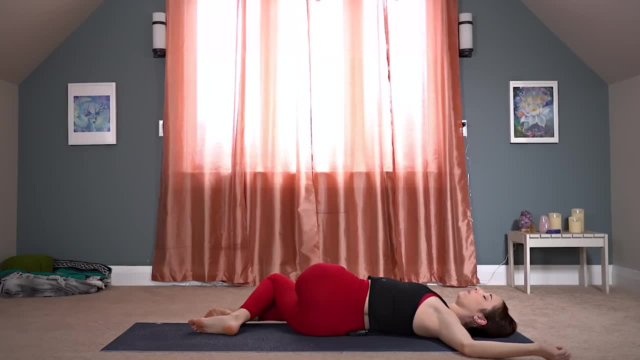 five breaths here, you and one more big inhale and let's lift back up and across your legs and it might feel good just to let your knees drop them side to side and windshield wiper motion coming into shavasana. you might wanna do this with the tradition way with your legs. 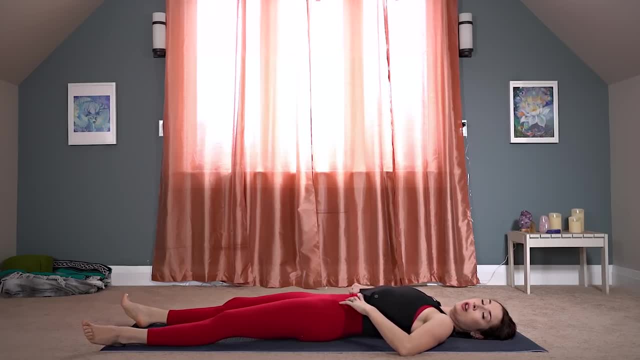 out in front of you. if you are experiencing tension in your lower back, sometimes straight legs aggravates it. if you are feeling tension in your lower back, sometimes straight legs just aggravates it, so you can widen your feet and just let your knees fall in towards one another, placing your arms. 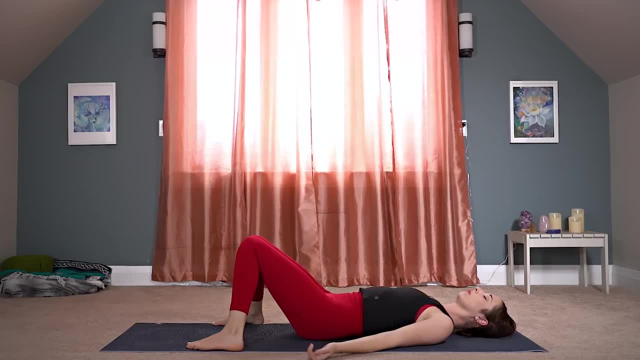 wherever is comfortable taking our last few moments of stillness. we'll take 10 slow, deep breaths right here. really important not to skip shavasana. this is your body's opportunity to really integrate all of the work that you've done. the worst thing we can do is to rush out. 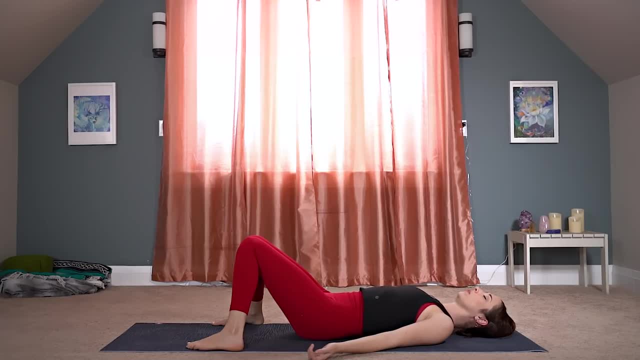 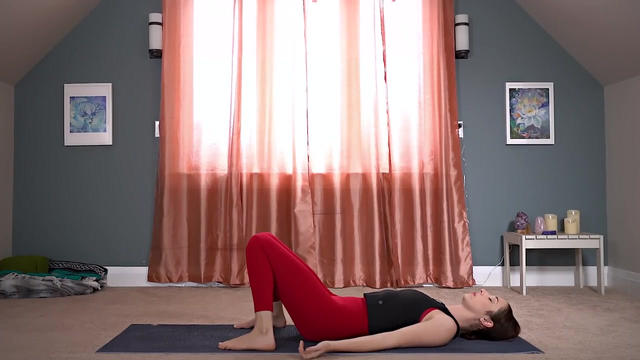 so just relax and breathe. here you start to deepen your breath to re-energize your body. wiggling fingers, it might feel good to reach your arms up overhead, to stretch out your legs out in front of you, and we'll roll to one side. push your hands into the floor to come up and take a seat. 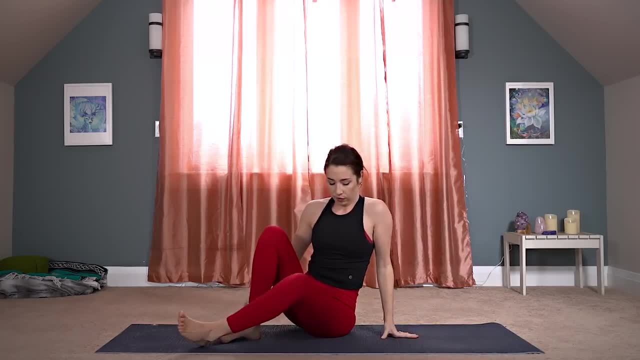 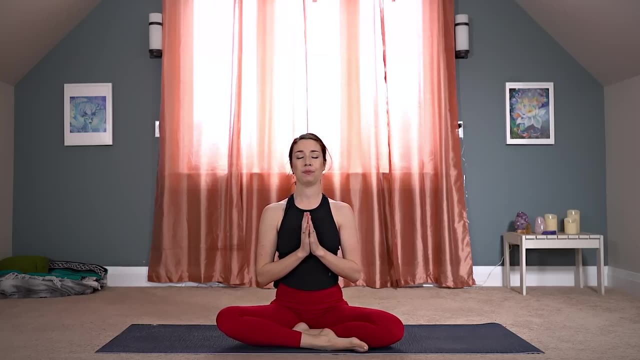 sitting in any way that is comfortable for your hips and your low back. we'll join our hands together at heart center. take a moment to really acknowledge the effects of your practice, noticing what's changed, what feels different now as opposed to when you first stepped onto your mat. 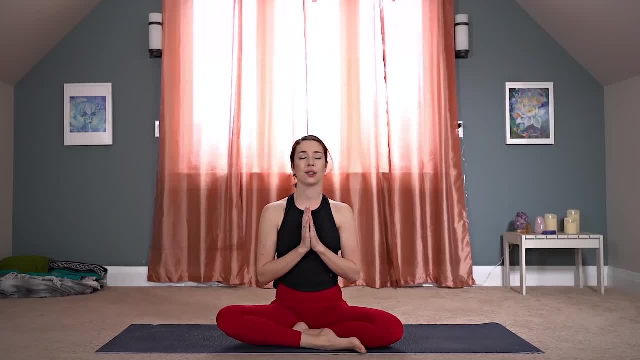 and we'll close our practice with the chant of om. one time let's inhale to chant big breath in namaste. thank you so much for doing this therapeutic practice with me. i hope you're able to notice some differences in your hips and in your low back. 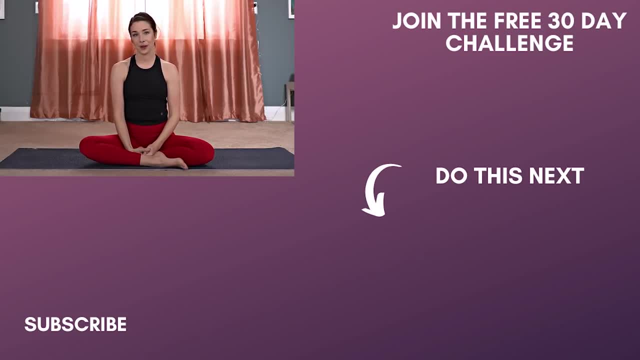 please leave me a comment down below. let me know how this went for you, and if you'd like to stay a little longer, you can follow this class up with this five minute meditation right here. i'll practice again with you soon, namaste.